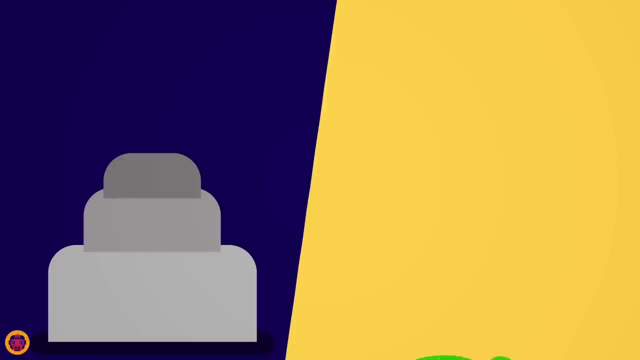 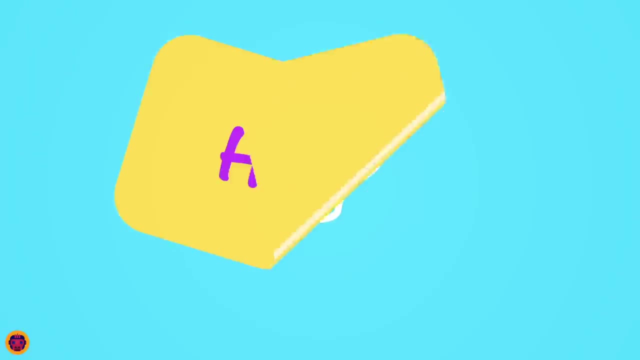 The knowledge stands still like a stone instead of growing and changing like a tree. So I started asking questions. I found that when someone makes a claim that something is true, the best way to test that truth is to ask a series of challenging questions. 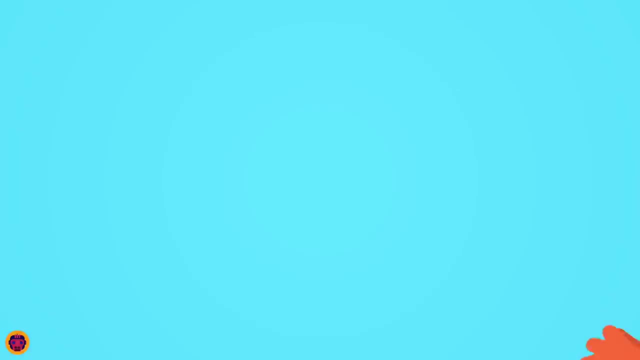 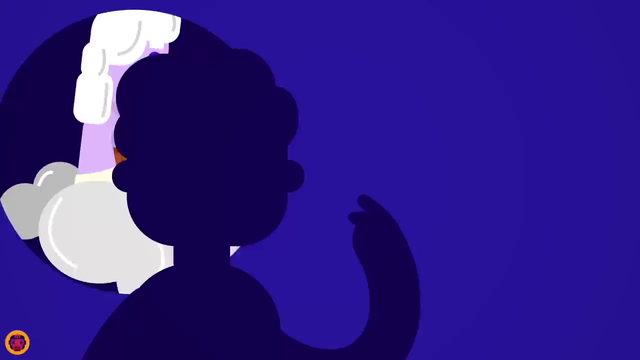 For example, if a man claims that it is virtuous to love the god Zeus, I would ask: what is virtue? What is love? Are there other gods to love? If they cannot even explain what virtue is, how can they say that it is virtuous to love Zeus If they cannot explain what love is? 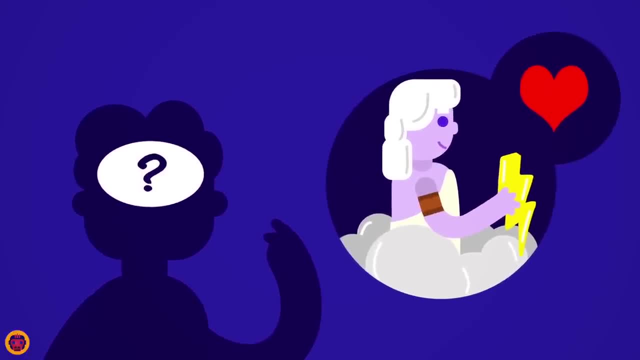 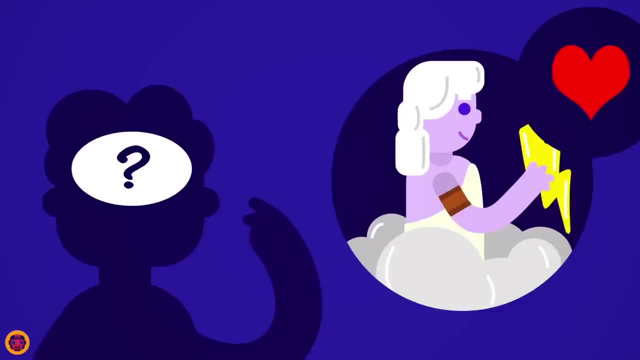 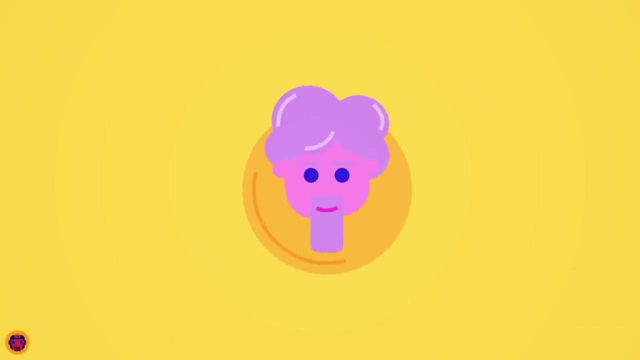 how can we know if we are really loving Zeus and therefore that we are virtuous? If someone making these claims cannot answer these challenges, then how can they know the truth of their claim? In my life I didn't publish any work, so write much down for others. 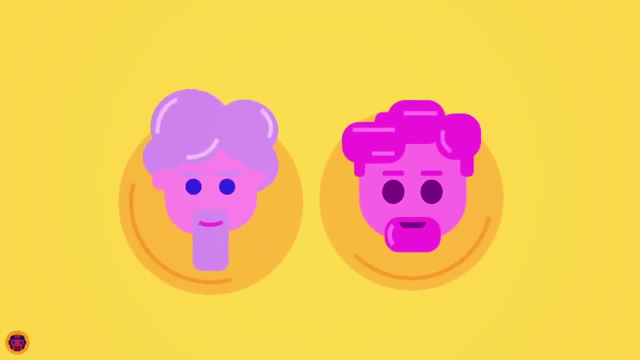 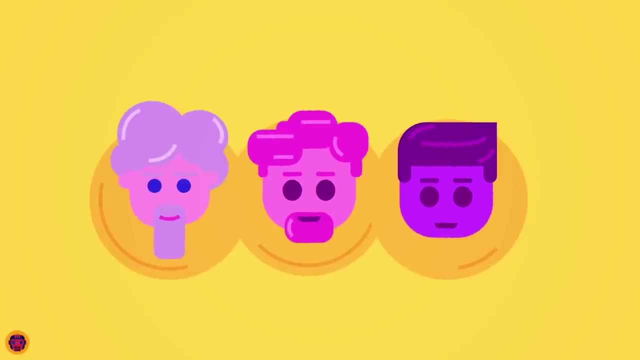 to read, But many young men in Athens, including a very bright student named Plato, used to follow me around and watch closely as I questioned some of the wisest men in the city. Plato would eventually pass this method down to his student, Aristotle, who was the two. 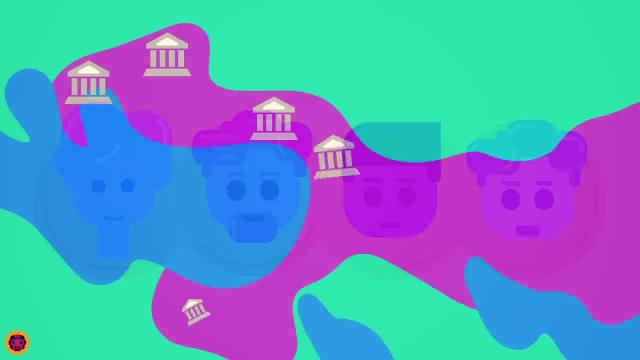 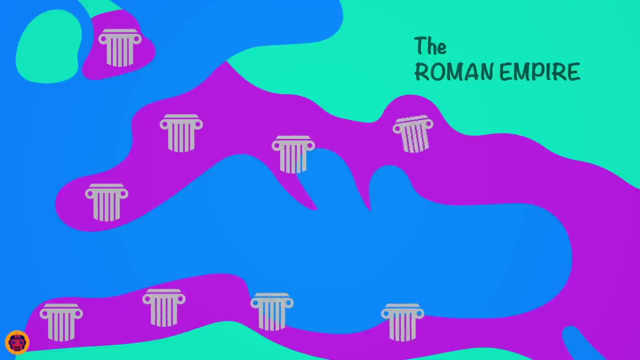 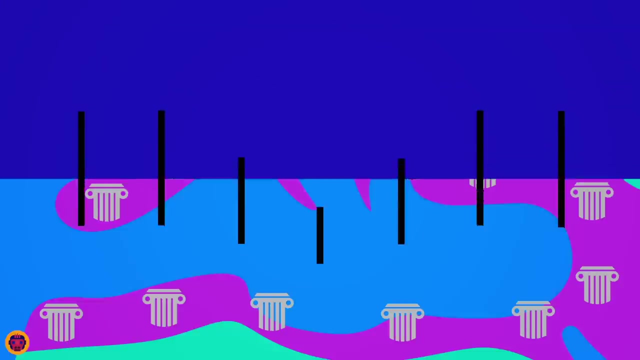 of Alexander the Great Alexander spread Greek thought to his vast kingdom. When the Romans took over Alexander's empire, they expanded it even larger and spread the Greek tradition even further. Sadly, when the Romans fell, the world entered a long dark period. 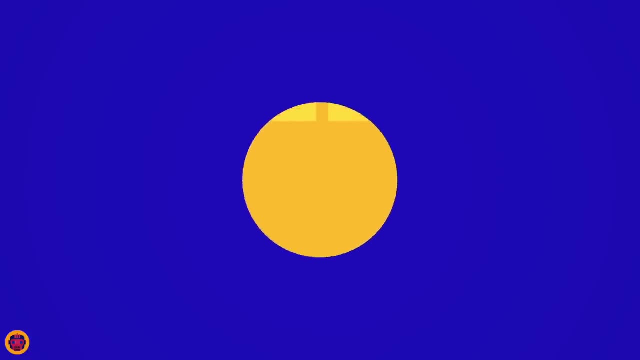 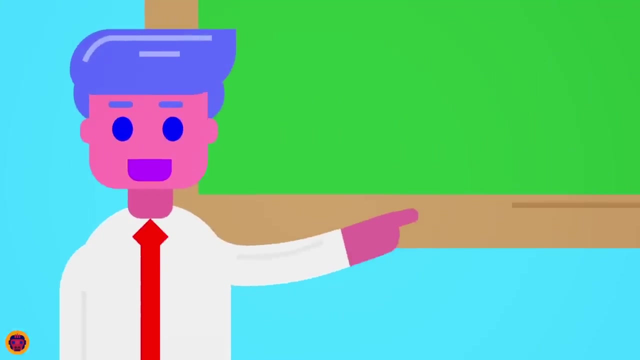 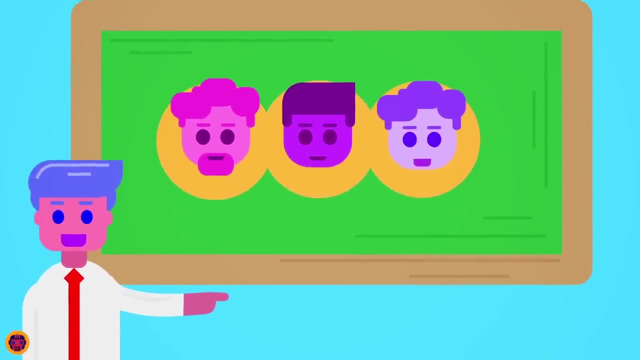 where knowledge stood still once again. But then something wonderful happened: There was a renaissance of thought and knowledge When people began to revive the works of my students. science flourished when people realized the power of methodical questioning and testing of claims. 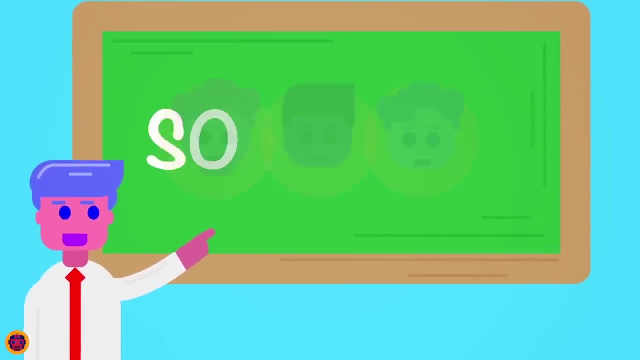 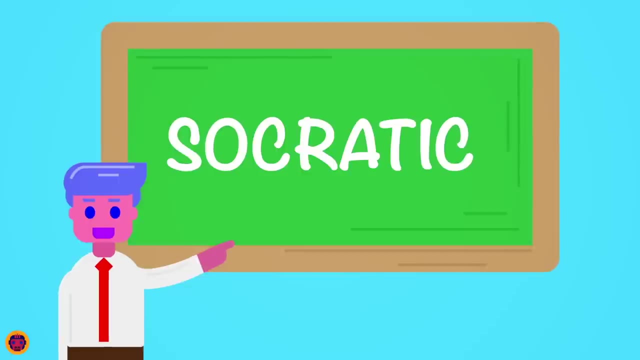 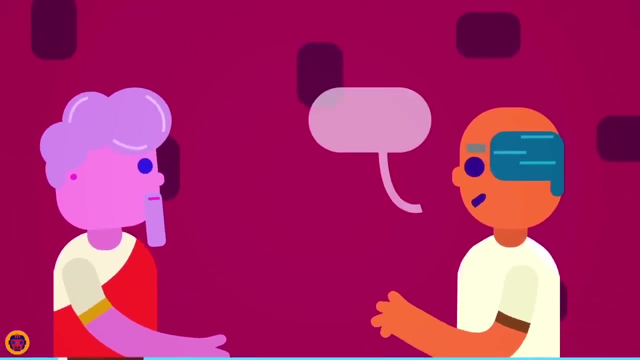 In your time. my method of questioning is known as the Socratic after me method and is the basis of modern scientific and philosophical inquiry. And all this because I asked a few questions. Many people think that when someone asks a question, 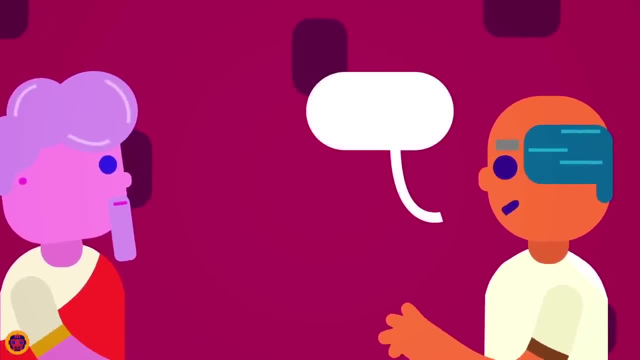 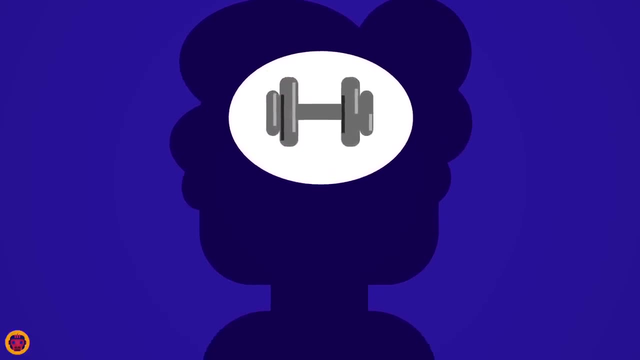 or many questions like I do, that they are unwise, But I think just the opposite. True wisdom is the knowledge of how little you actually know. It is this realization that allows you to start asking questions and get to the real truth.